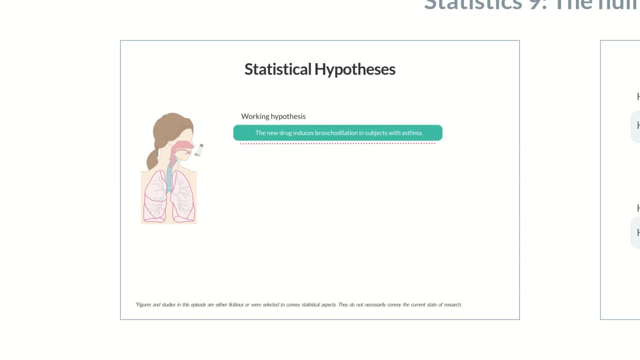 suitable for conducting a study because it's too general and therefore harder to test. So which variables should be used to assess the drug success, and what should the study measure? Now the pharmaceutical company decides to perform pulmonary function tests to assess potential bronchodilation. Specifically, they decide to use the change in forced expiratory. 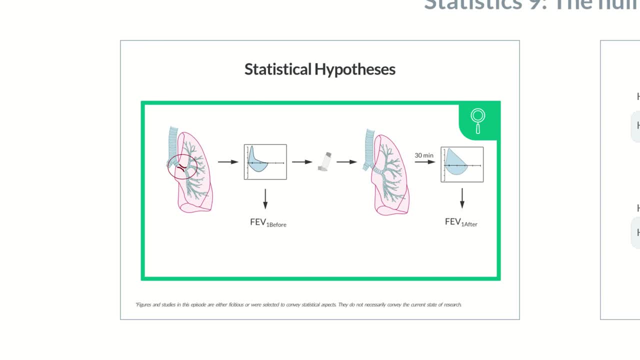 volume in one second. Introduction of the new drug induces bronchodilation in subjects with asthma. The diagnostic hypothesis as FEV1 before and 30 minutes after taking the drug. From the difference between these two values, the change in the volume of air forcibly expired. 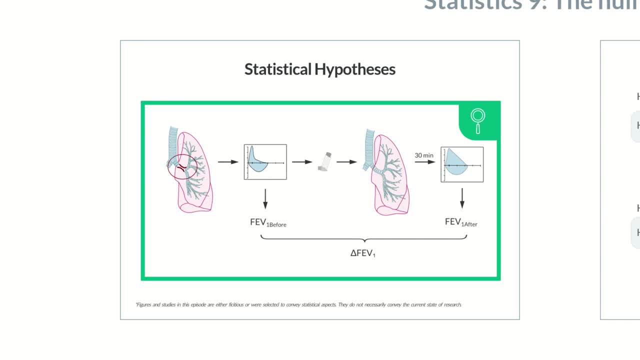 in one second is measured and therefore can indicate a potential decrease in obstruction and effective bronchodilation. If you'd like to find out more about pulmonary function tests, check out our Chalk Talk episode on spirometry, where we explain what the FEV1 value is and how to determine it. 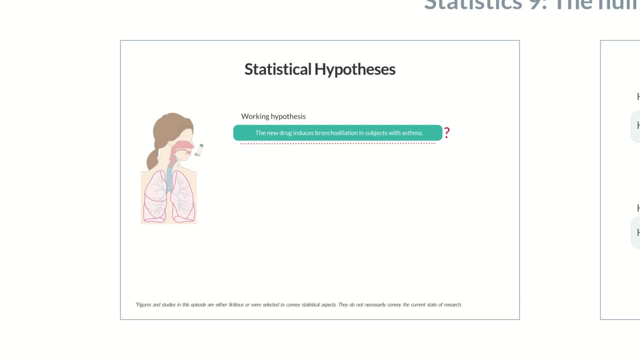 Now the working hypothesis can be formulated more specifically. In test subjects with asthma, the amount of air expired in one second changes 30 minutes after administration of the drug. With this alternative hypothesis we have an assumption of what to observe in the study. 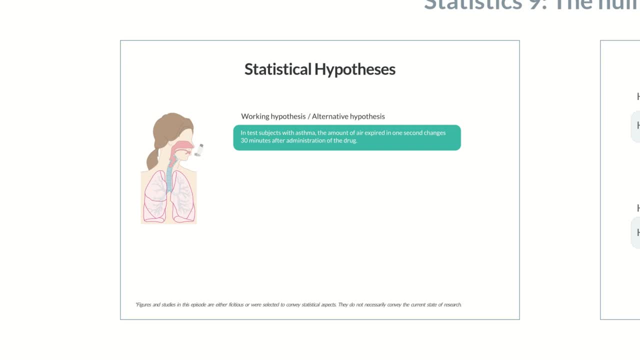 and what outcome to expect. However, the alternative hypothesis is still nonspecific because it doesn't specify the size of the expected change, nor does it rule out a decrease in FEV1. Although it's unlikely, Without detailed prior knowledge, a more specific hypothesis can't be formulated. 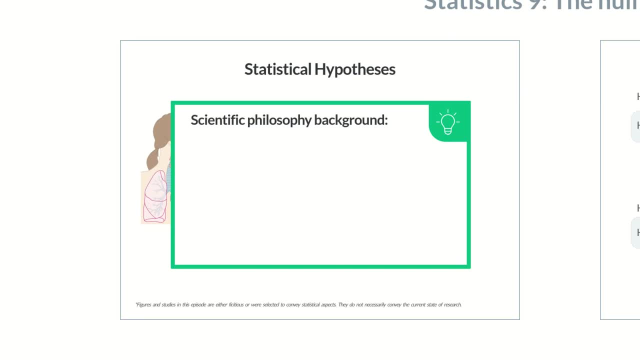 To avoid the predicament of a lack of prior knowledge, a strategy derived from the philosophy of critical rationalism can be applied, In other words, acquiring knowledge through contradiction In this approach, which can be traced back to the scientific philosopher Karl Popper. 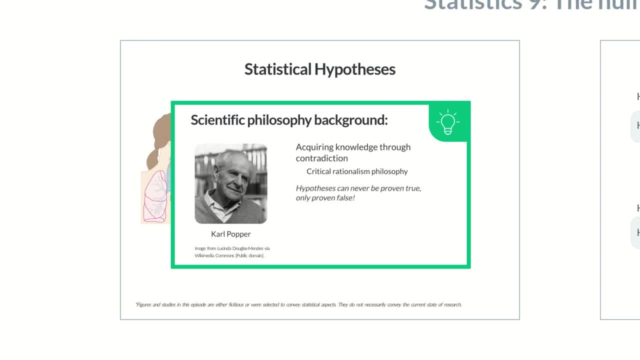 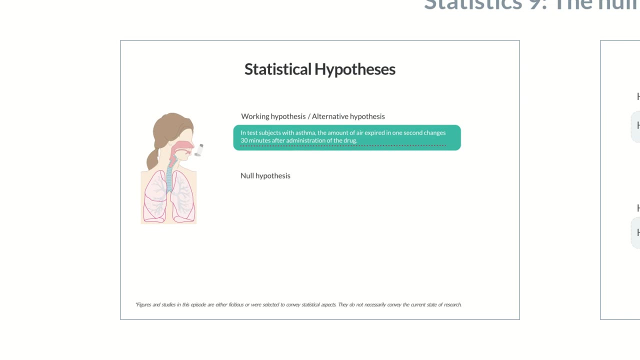 it's assumed that hypotheses can never really be proven true, only be proven false. In this theory, the validity of a hypothesis is demonstrated by showing its opposite is false. So instead of the alternative hypothesis, the null hypothesis is tested in statistics. The null hypothesis is mutually exclusive to the alternative hypothesis. 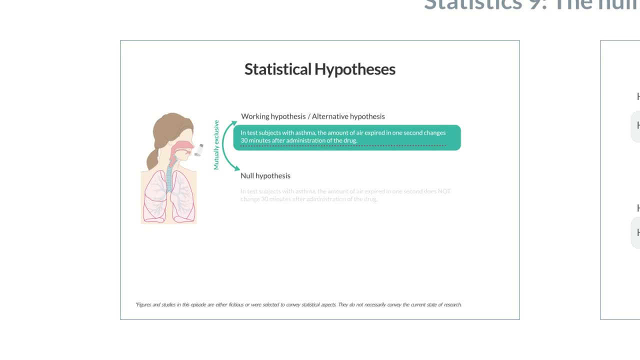 So in our example the null hypothesis would be: in test subjects with asthma, the amount of air expired in one second doesn't change 30 minutes after administration of the drug. in other words, there's no observable difference in FEV1 on administration of the drug in test. 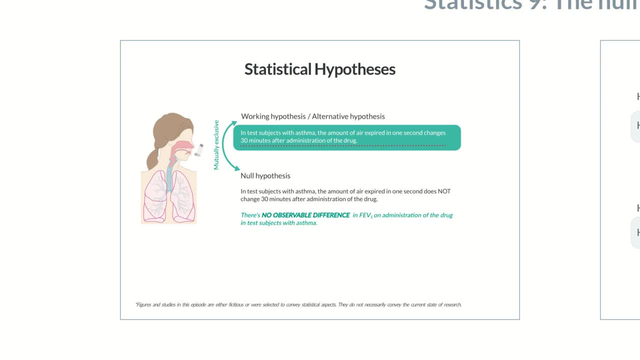 subjects with asthma, Because both hypotheses can't be correct at the same time. the working hypothesis is the alternative to the null hypothesis. By the way, there's also an abbreviation for the null hypothesis H0, and for the alternative hypothesis H1. 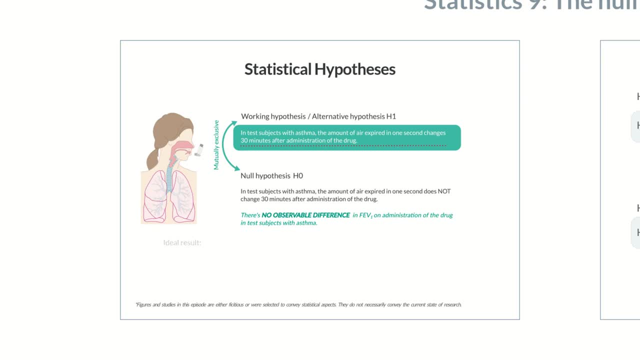 If a study is conducted using the null hypothesis, the result should ideally show that the observations are incompatible, So the study should falsify the null hypothesis. According to Popper's theory, the alternative hypothesis is assumed to be true without it needing to be analyzed. 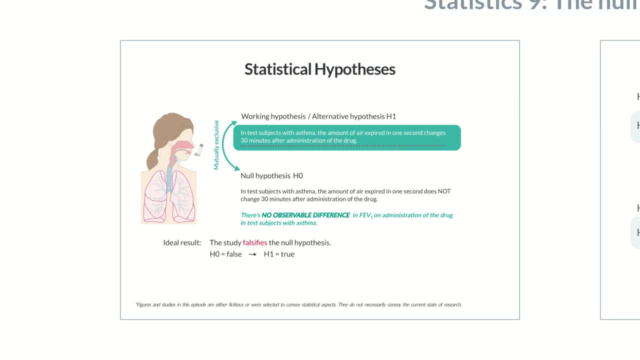 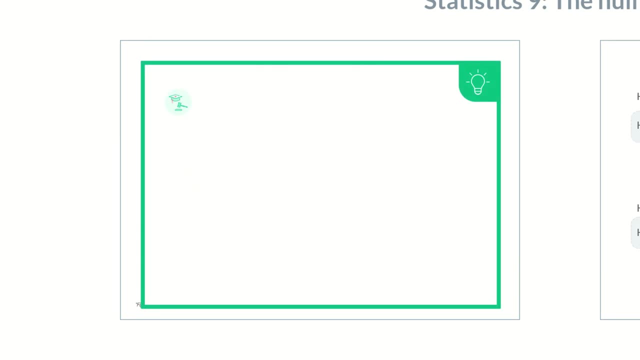 Does indirect verification seem somewhat odd? In fact, you probably know this procedure from another application, namely in criminal trials. In court cases, the alternative hypothesis is: the defendant is guilty. Accordingly, the null hypothesis is… The defendant is not guilty. 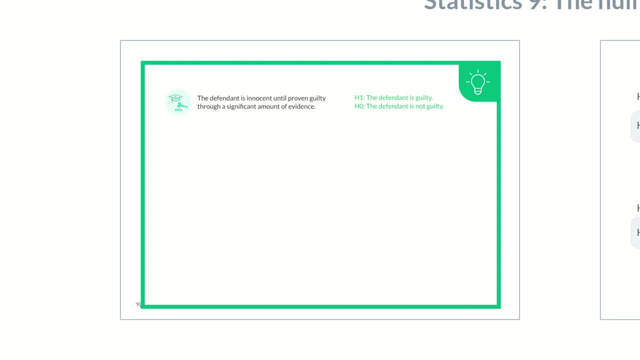 Court proceedings should prove that the null hypothesis is false. Courts are required to consider the defendant as innocent until proven guilty with a significant amount of evidence. In statistics, the same approach applies. The null hypothesis is considered true until the sample data shows otherwise. 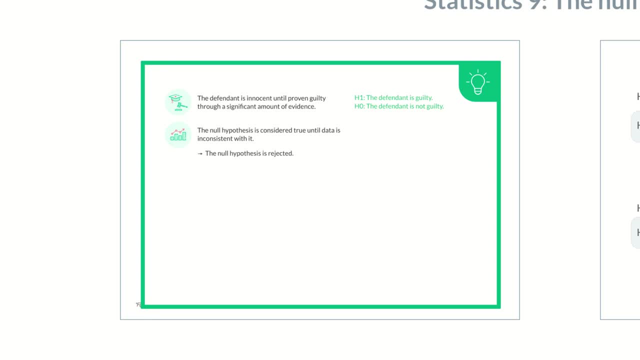 In this case, the null hypothesis is rejected and its mutually exclusive alternative hypothesis accepted. This indirect approach via the null hypothesis can be initially confusing, especially because study data is usually published as though the alternative hypothesis was analyzed, not the null hypothesis. Often, the null hypothesis isn't mentioned in publications. 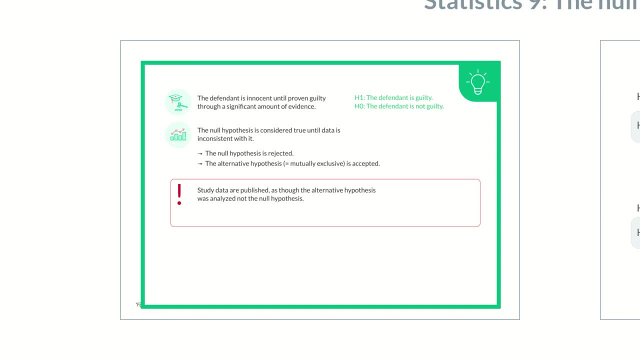 In clinical studies. clinical evidence usually indicates that a drug leads to substantial improvements. However, the study actually only provides evidence that the drug alters the measured variable. The drug is not the result of the analysis. The positive or negative effect is initially not so important. 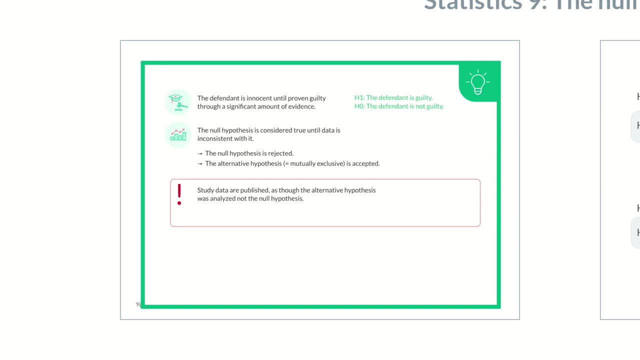 Theoretically, a study can also be considered significant if the drug demonstrates a clear disadvantage for the participant. Now how is a null hypothesis correctly formulated? First, it's important to know what the term- the null hypothesis is mutually exclusive to the alternative hypothesis- means.